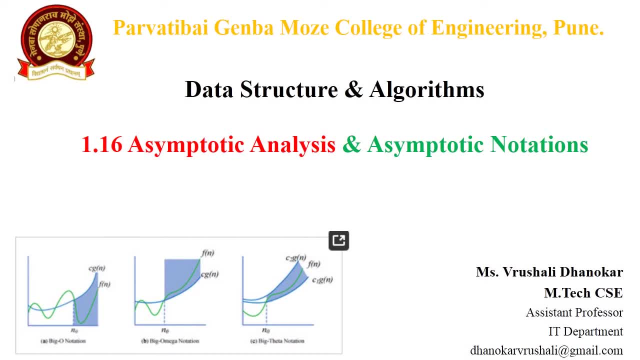 Good morning everyone. I am Rishali Dhanogar, Assistant Professor, IT Department. In my last video, we learned about space complexity, time complexity of the algorithm. Now, in this video, we will learn about asymptotic analysis and asymptotic notation. So let's. 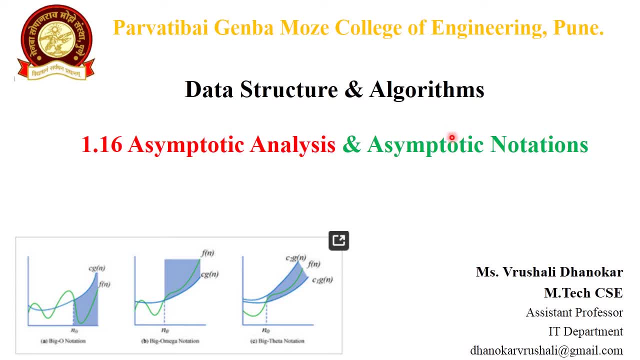 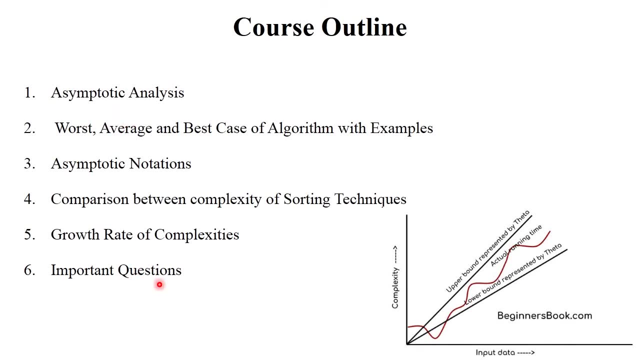 see what is meant by the analysis and their regarding notations. Next, following points are covered in this video, which includes asymptotic analysis, worst, average and best case of algorithm with examples, then asymptotic notation, the comparison between complexity of sorting techniques, growth rate complexities and important questions. So let's see one. 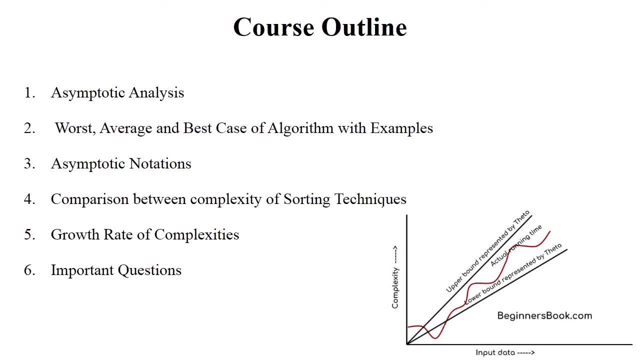 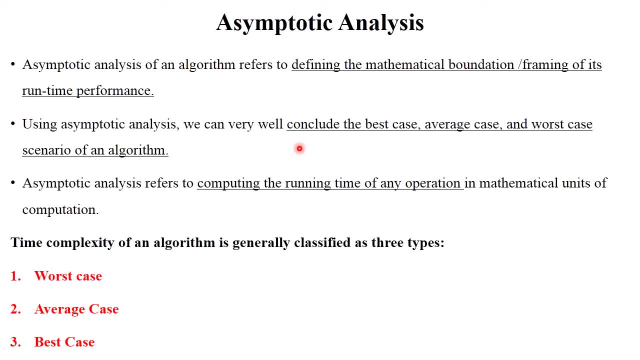 by one. what is meant by asymptotic analysis? So in my last video we discussed about space complexity and time complexity. So denotion of time complexity or time complexity is declared by asymptotic notation or the analysis. Asymptotic analysis of algorithm refers the defining, the mathematical boundary or framing of its. 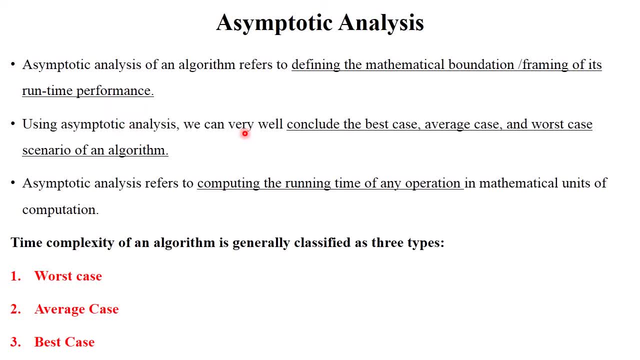 runtime performance. Asymptotic analysis very well conclude the best case, average case and worst case scenario of algorithm. Asymptotic analysis refers the computing running time of any operation in mathematical units of computation. So asymptotic analysis. it can be classified into the three. 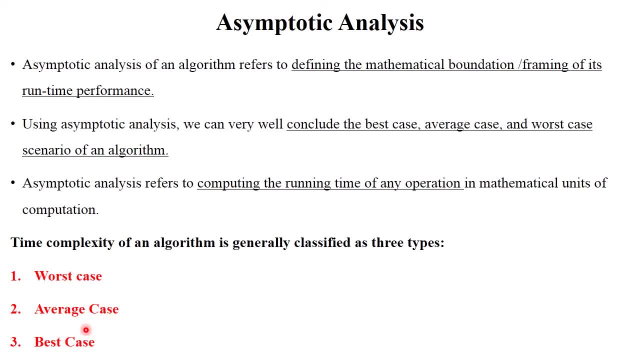 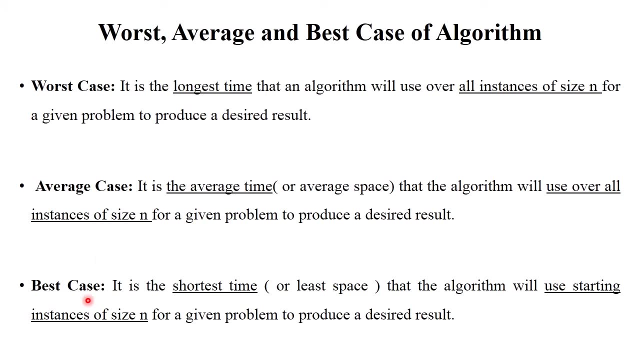 types: worst case, average case and best case. This case is regarding to the time complexity of your algorithm, So let's see, one by one, what is meant by worst case Next. So here there are three types of asymptotic analysis: Worst case, average case and best. 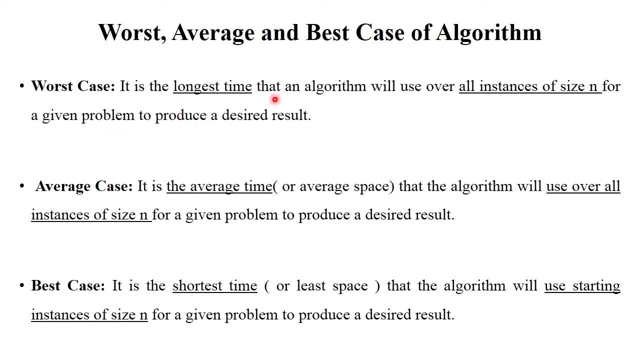 case. Worst case means it is the longest time of an algorithm. If the particular algorithm required longest time for solving the particular problem or declare the result, So this longest time is denoted as a worst case of that particular algorithm. It will use over all instance of. 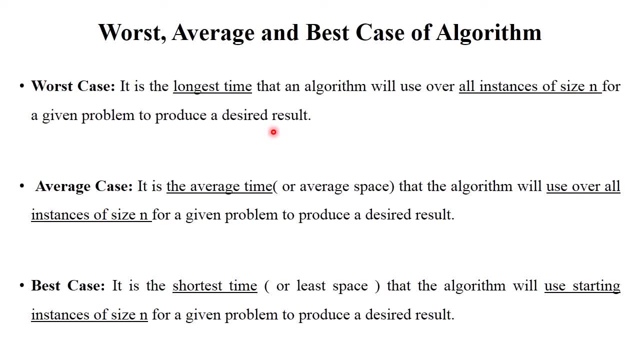 size n for a given problem to produce a desired result. I will explain through with example in my next slide. The next one is average case. If the particular algorithm required average time, not short or not longest in between, that is average time of that particular. 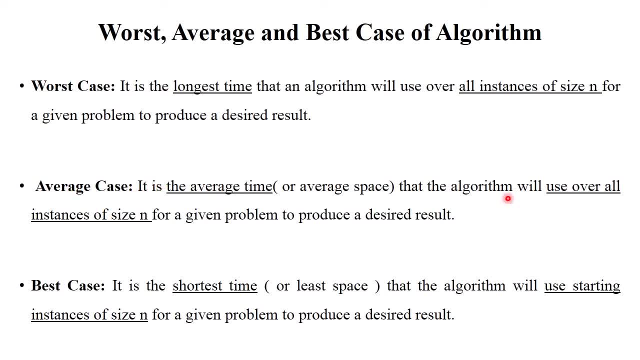 algorithm which is declared by the average case. we use over all the instance of size n for a given problem to produce the desired result, And the last one is best case, So if algorithm required shortest time to solve the particular problem or to declare the result, 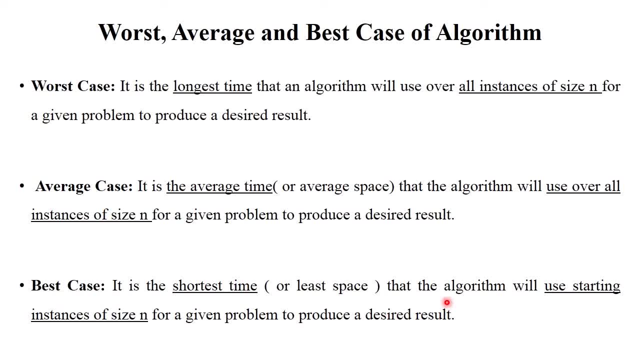 then this analysis is known as best case. That algorithm will use starting instance of size n for a given problem to produce the desired result. So concept of worst case means find out the longest time of algorithm. Average case means average time required to the algorithm. 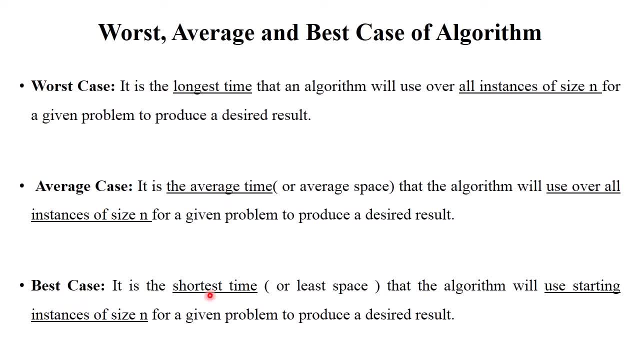 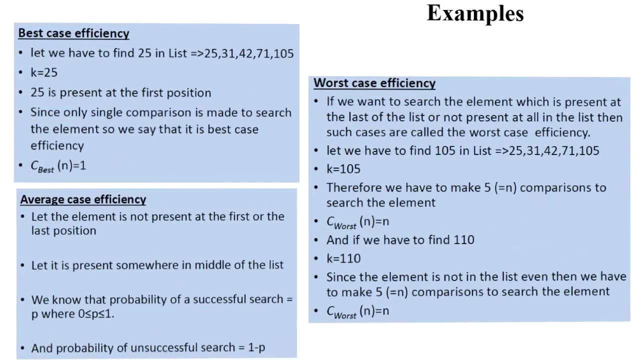 And best case means shortest time or minimum time is required for the algorithm to solve the problem. Clear, This is just concept of worst case, average case and best case. So I will explain through example in my next slide. So see here. these are the examples. 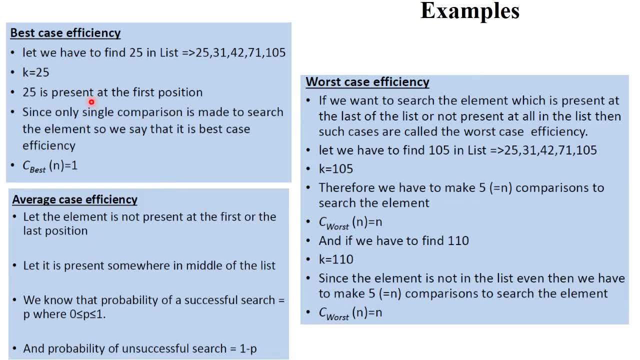 of best case, worst case and average case. Let's take first example here. Suppose we have to find out 25 in the given list. I already explained in my previous video about linear search algorithm, binary search algorithm and other sorting techniques. Hope you have. 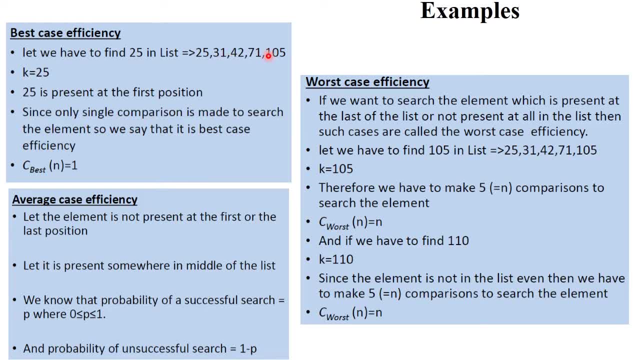 watched my previous video, So see here: the given input is 25,, 31,, 42,, 71 and 105.. And you have to find out 25 in the list, So searching element is 25.. So you have to start the comparison. 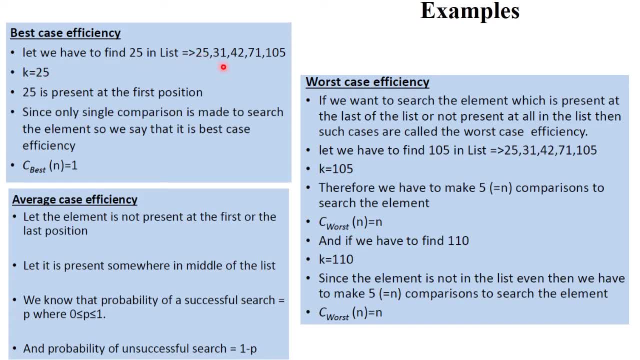 from the first element in that particular array or the list. Okay, So you have to compare 25 with the first position element, that is, 25.. So 25 is compared with 25.. So 25 is present at the first position, So it only requires. 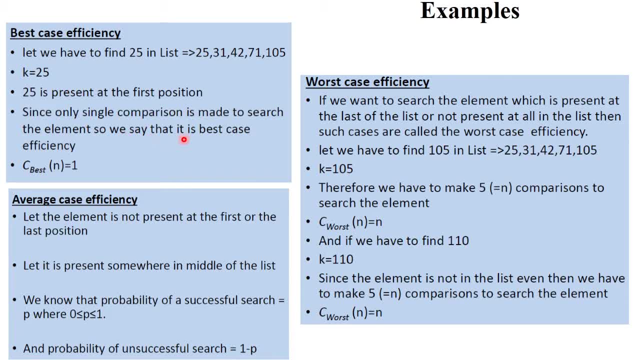 single comparison to make the search the element. So we have to say it is a best case efficiency. Right On the first comparison you got your element or the searching element, So it requires minimum time. Only one comparison is there, So this is called as best case efficiency. 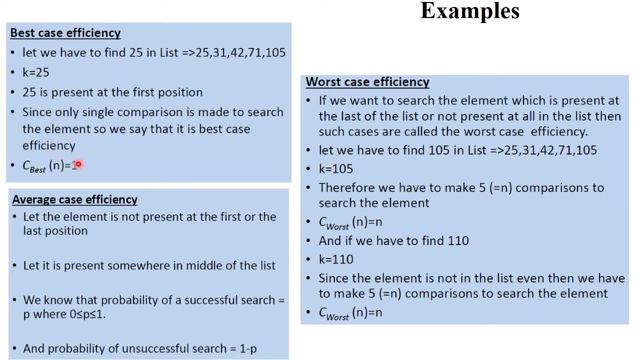 Clear. This is the example of best case. Best case efficiency is already denoted as 1.. That is n of 1. Means constant time or minimum time is required for the algorithm Clear. The next one is worst case efficiency. If you want to search, 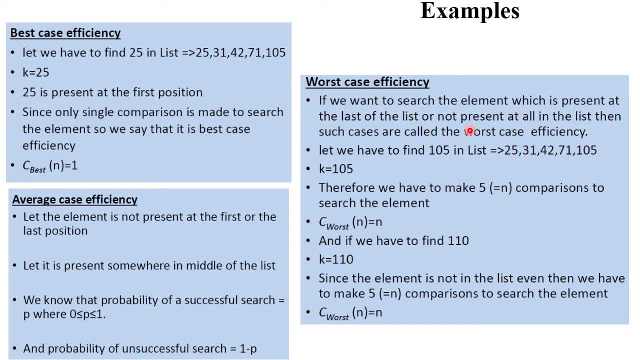 the element which is present at the last of the list or not present in the list, then such cases are called as worst case efficiency. Let's take this example: Suppose the given input is 25,, 31,, 42,, 71 and 105. And you have to find out one search element. So 25 is. 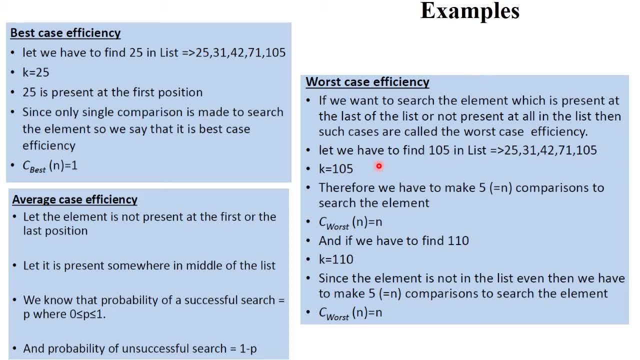 present at the last of the list and that element is present at the last of the list. What is the search element? This is the search element. So you have to find out 105,, this element in the list. This is your searching element. So you start the comparison with. 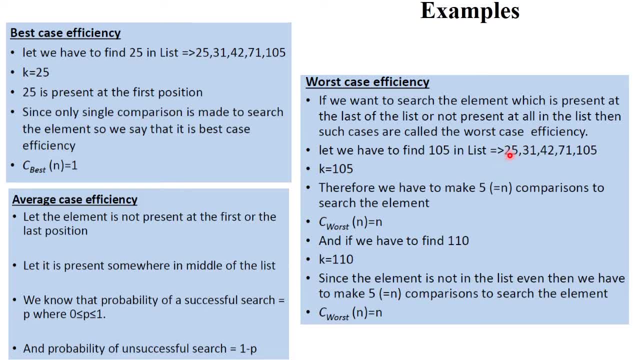 the first element. in linear search algorithm, 105 is compared with 25, not found. 105 is compared with 31, not found. In this way you have to compare each and every element in the list linearly upto the last element. So we have to find out 105 at the last location. 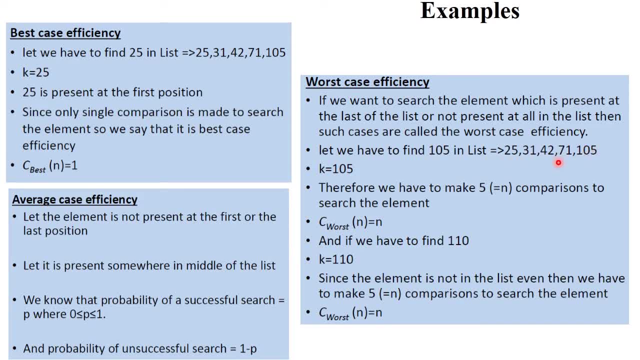 of that particular given input. Right … Means… It means it required maximum time, because 105 present at last location means it requires n number of comparisons. right, How many comparisons are done? 1, 2,, 3,, 4 and 5 means there are total n comparisons are required. 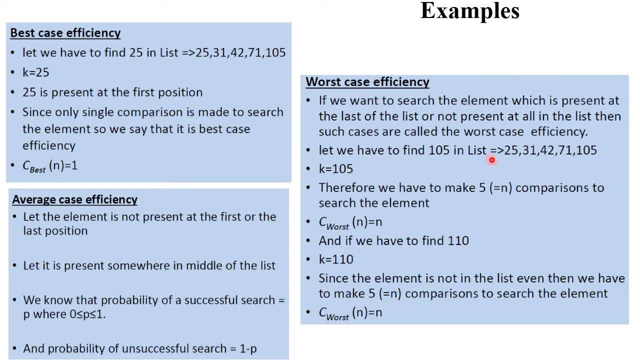 This is called as worst case means it requires maximum time for solving the problem. clear. And the second case in worst case is if the element is not present in the list. Suppose we have to find out 110 in the given list. Again, we start the comparison from the first location. 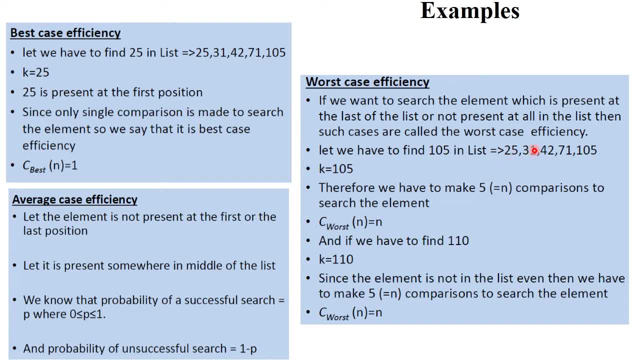 110 is matched with 25, not found. Again, matched with 31, not found. In this way we have to start comparison one by one, linearly and up to 105.. 105 is the last element, So 110 is not present in the list. 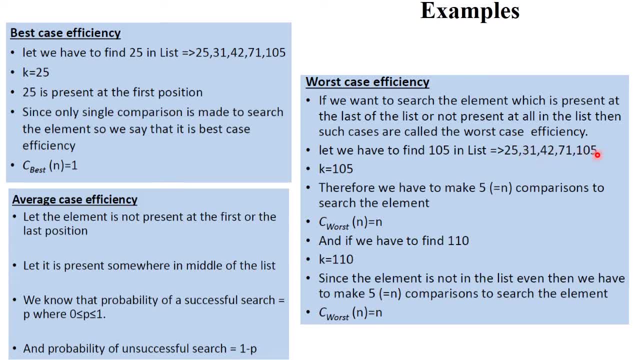 At that time. also, n number of comparisons are required there. clear. So these two cases- Last location and elements- are not found. This case are involved in worst case efficiency. clear. So this complexity is denoted by the n okay Means n number of elements you have to compare. clear. 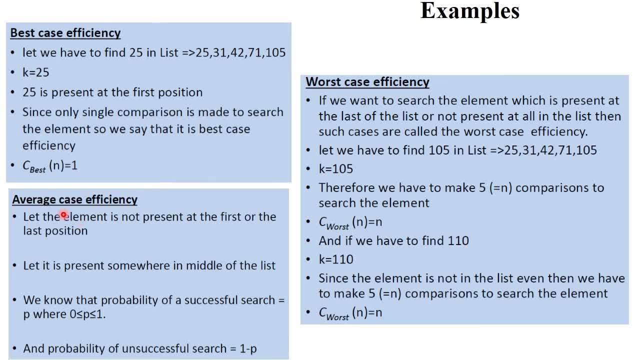 This is called as worst case And after that there is average case, efficiency Let: the element is not present on the first location And also element is not present on the last location. It means that element is present somewhere in middle of the list. 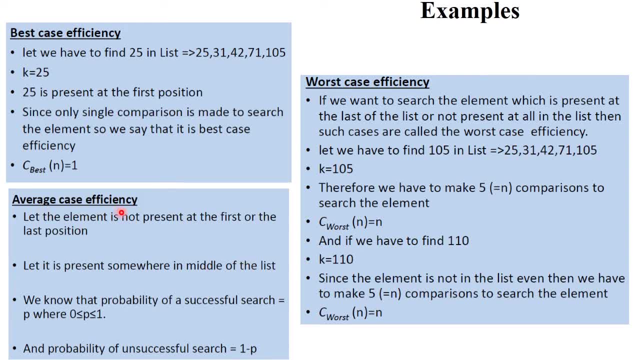 This is called as average case efficiency. clear: Suppose you have to find out 42 in the given list. So 42 is present in middle of that particular list: 31,, 42 and 71. If we find out this element in that given list, so this is called as average case efficiency. 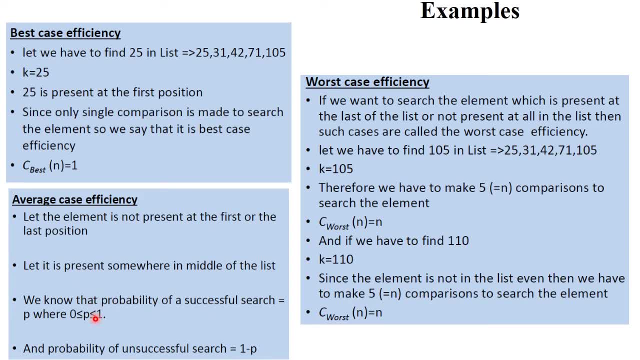 So we know that probability of successful search is between 0-1.. Means if element is present in between first to last location, Means this is called as successful search okay. And if the element is not present in the list, this is called as unsuccessful search. 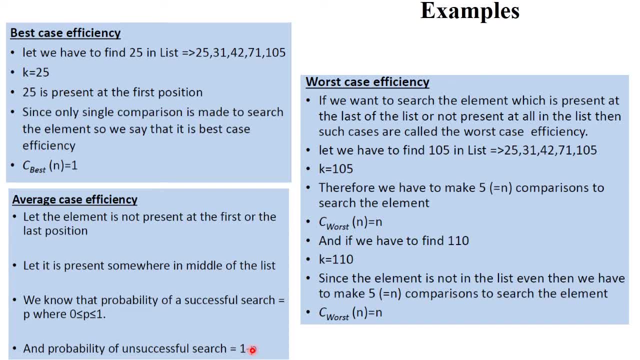 Which is also denoted by 1-p. okay Means you have to search complete input and your element is not present, Which is denoted by 1-the probability clear. So these are the example of best case, worst case and average case. 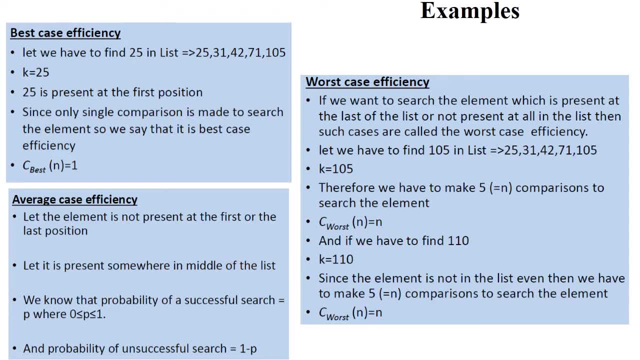 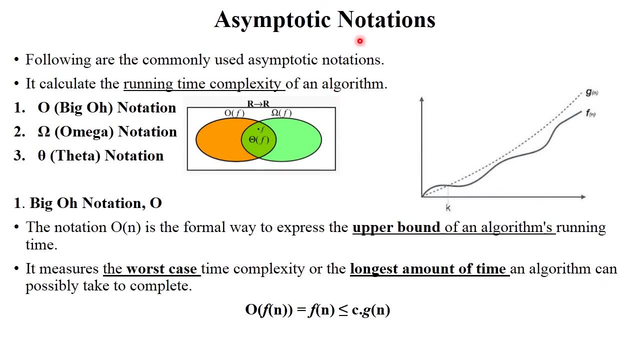 Hope so you understood the introduction of best, average and worst case. Next. Next topic is asymptotic notation. Following are commonly used asymptotic notation. Asymptotic notation calculate running time. complexity of algorithm: See. there are total 3 asymptotic notation. 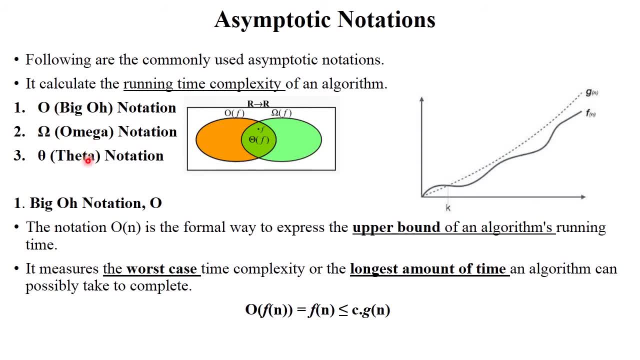 That is big O, omega and theta notation. Big O is declared as on that This is called as big O, this is called as omega and this is called as theta notation. clear. These are the 3 notations, So let's see how it will be used. 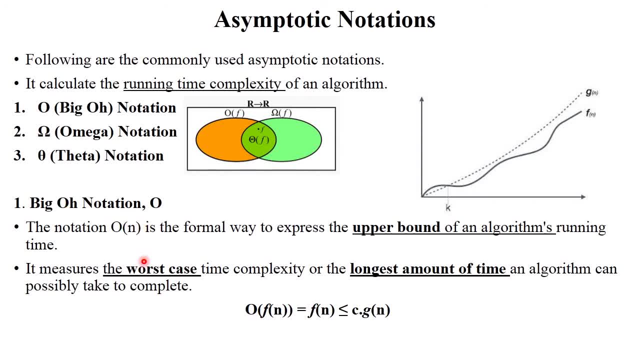 The first one is big O notation. okay, I already explained in my previous slide. worst case time complexity right. Worst case means element is present at the last location on that, given input Means it required maximum time to solve the particular algorithm right. 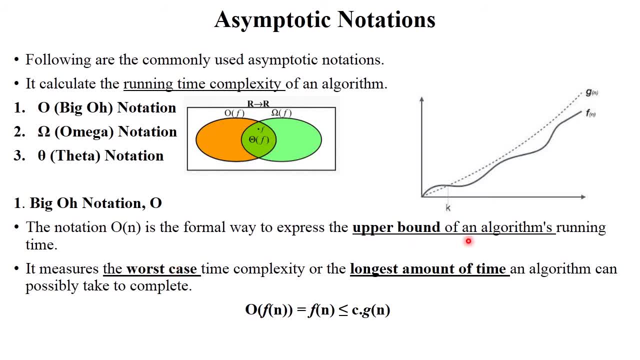 So big O and notation are the same. The second one is express the upper bound of an algorithm, or running time complexity. Upper bound means last location. It measure the worst case time complexity of the longest amount of time algorithm can possibly take to complete. 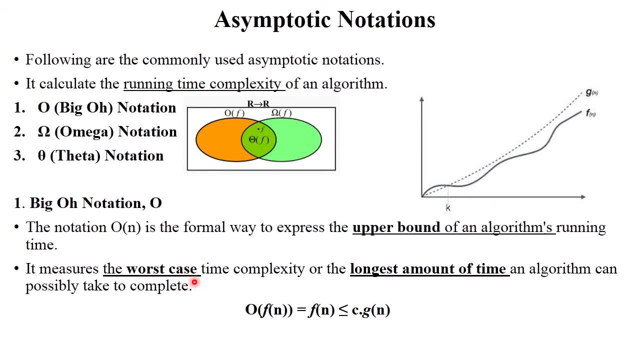 If your algorithm required worst case, then it will be denoted by big O notation, clear See in this diagram. this is just a structural way. This is your given input And this is the time complexity. There are 2 functions are used: f of n and g of n. 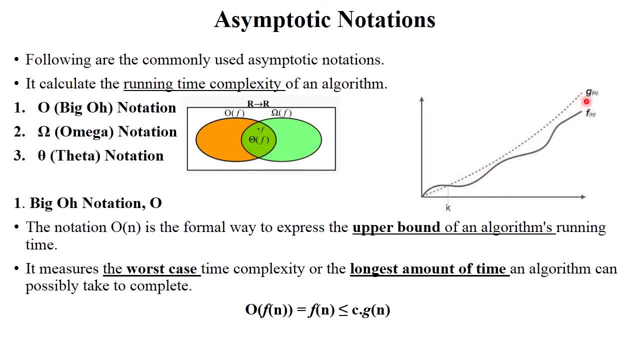 f of n indicate your given input- okay. And g of n indicate the time complexity or worst case time complexity of your algorithm. This is called as upper bound Means. it required maximum time for solving the particular examples. clear. So big O notation is used for worst case time complexity- clear. 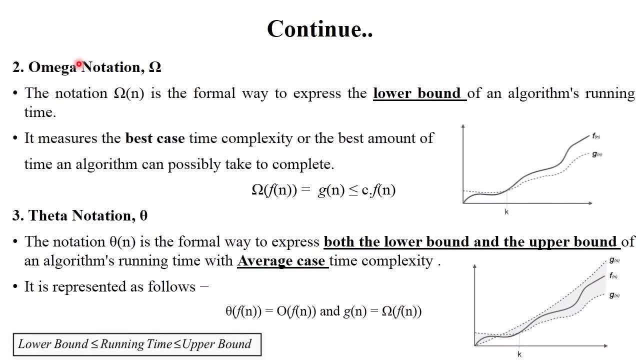 Next. The next one is omega notation. The omega notation is express the lower bound of an algorithm running time. It measure the best case time complexity of algorithm. What is mean by best case? Best case means element is found at the first location in the given input right. 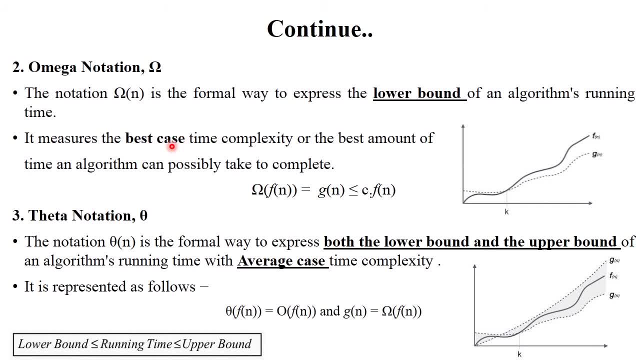 Means. it requires minimum time to solve the particular problem, right? So best case is denoted by the omega notation. See in this diagram: The g of n is your given input and f of n means lowest bound. okay, f of n is your given input size and g of n indicate the best case of time complexity. 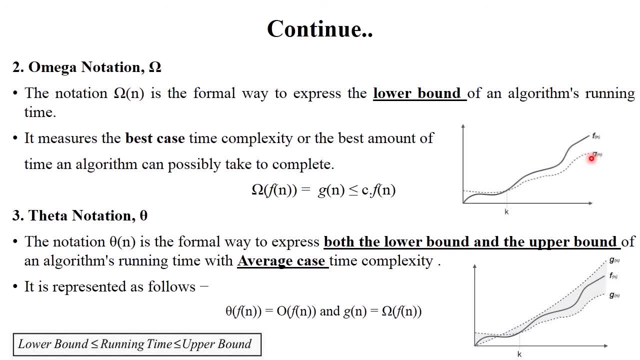 Means it indicates the lower bound right. It requires minimum time, So your time is less than your equation clear. The next one is theta notation. Theta notation denote the average case. Average case means middle of that particular given list. So theta notation express both lower bound and upper bound of that particular algorithm right. 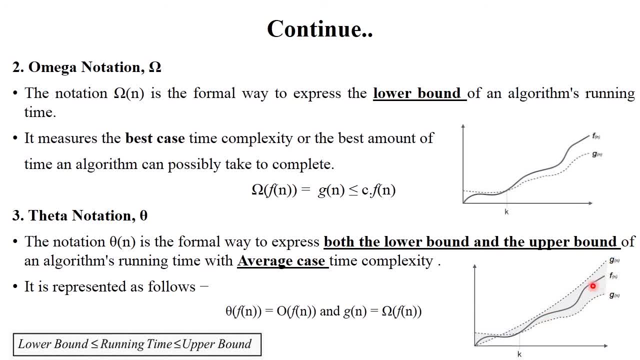 See here In this diagram. This is your given input: f of n, okay, g of g1 of n and g2 of n means it indicates best case, It indicates worst case and in between this there is average case of that particular algorithm. clear. 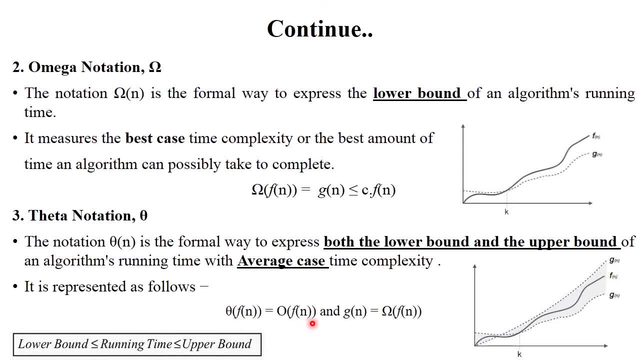 So f of n is equal to big O of f of n and g of n equal to omega n, g of n equal to omega of that particular equation. clear. So you have to remember What you have to remember. Theta notation means average case. 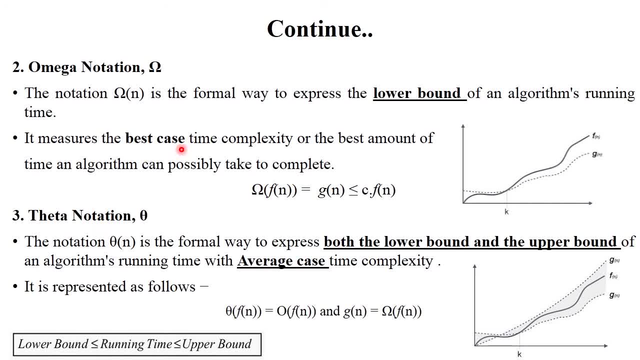 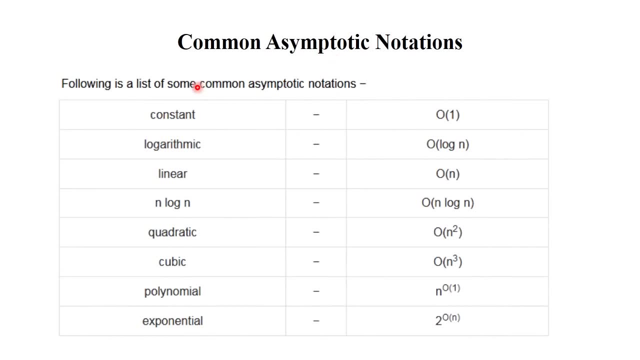 Average case denoted by the theta notation. Best case is denoted by the omega notation: okay, And last one is worst case is denoted by the big O notation, clear. Next. Now, these are the some common asymptotic notation. Here is the list of some common asymptotic notation. 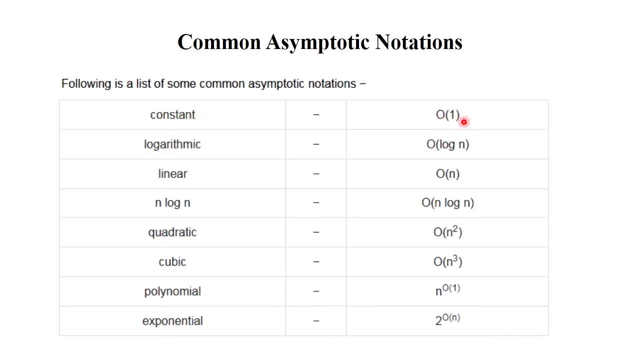 If your problem is required constant value, then your time complexity is big O1, okay. If there is logarithmic equations are present, then the time complexity of that algorithm is big O log n. If there is linear equations are present, for example linear search algorithm, right. 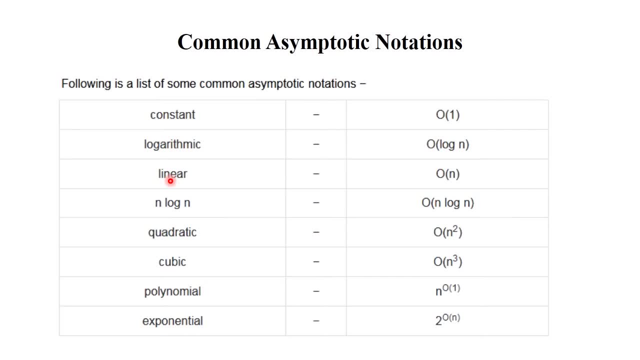 We have to compare from start to end each and every element. So it is denoted by big O of n n means number of inputs are present in the given list. Then n log n. n log n is generally used for divide and conquer technique. 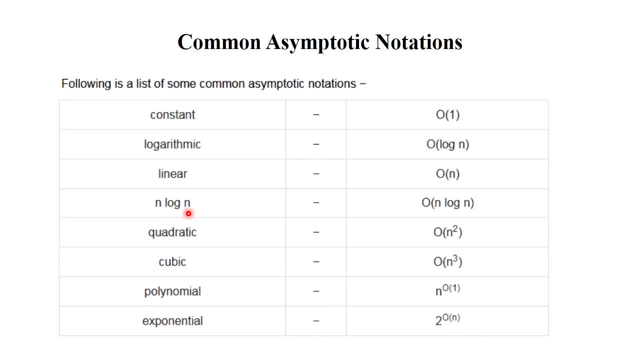 I already explained merge sort and quick sort in my last video. okay, So divide and conquer technique is represented by big O n log n time complexity If your equation present a quadratic format, so which is represented by big O n square And also the bubble, sort, selection sort, insertion sort. this technique also have the time complexity, big O n square. 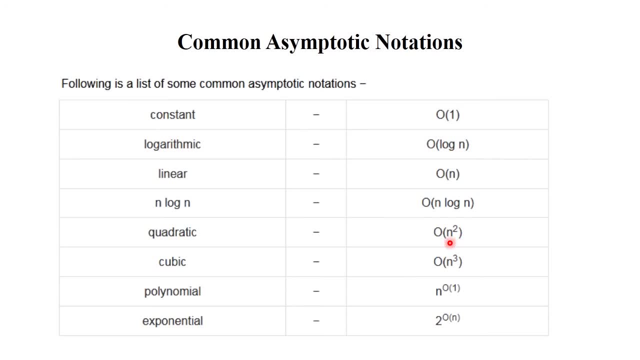 Because there are two elements, Means first element compare with second element. second element is compared with third element. like this Means there are two, for loops are used. So which is indicated by the big O n square. If your algorithm present some cubic element, so the time complexity of that equation is big O n cube. 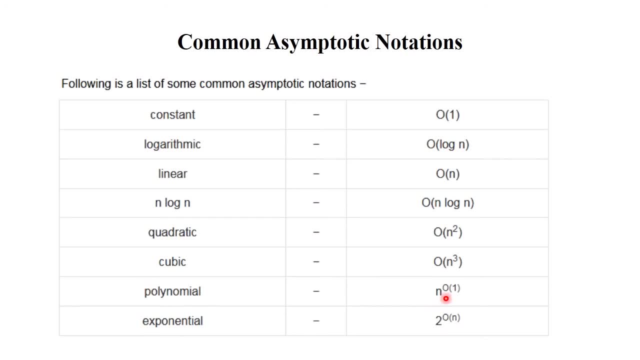 For polynomial equation: For polynomial equation, time complexity is big O 1 base n. And for exponential equation, the time complexity is big O n base 2.. Clear, These are the common asymptotic notations or, the worst case, time complexity of the algorithm. 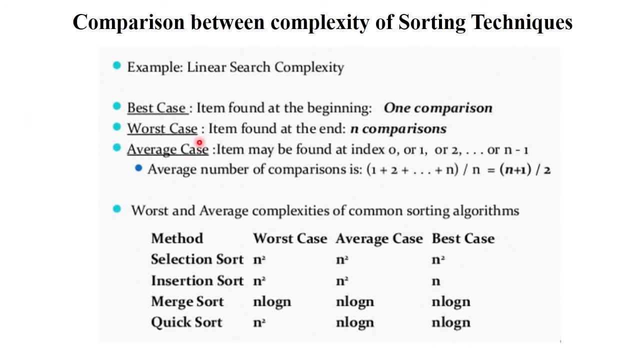 Clear Next. Now here is comparison between complexity of sorting techniques. Okay, Let's take the example of linear search complexity. I already explained Best case, worst case, average case. Best case means element found at the beginning. Only one comparisons are there. 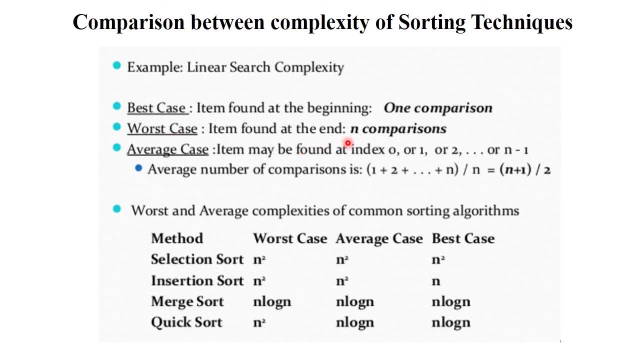 Worst case means element found at the end Means n number of comparisons are required And average case means elements are found at the index between 0, 1, 2 upto n-1.. Right, So worst and average complexity of common sorting algorithm are in this way: 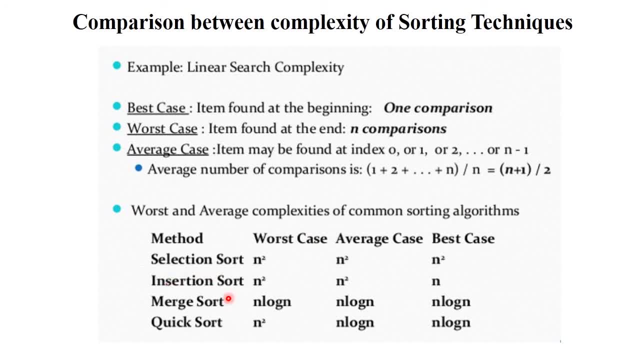 I already explained selection sort, insertion sort, Merge sort and quick sort. So it must or you have to remember this time. complexity of the algorithm. This is one of the most important part in data structure: The selection sort, the worst case time. complexity is n? square. 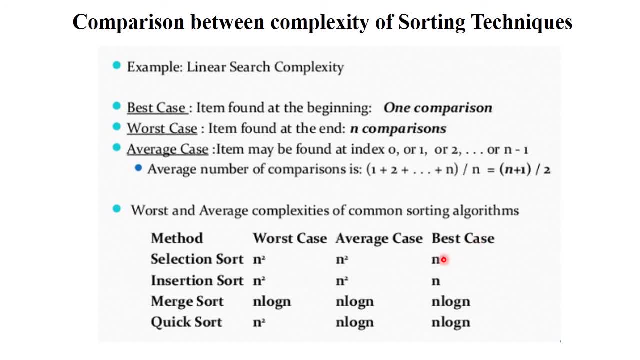 Average case is n square And best case is also n square, You have to just remember it. Okay And similar to merge sort is n log n all in worst, average and best case: Okay. And for quick sort, the time complexity of quick sort in worst case, n square. 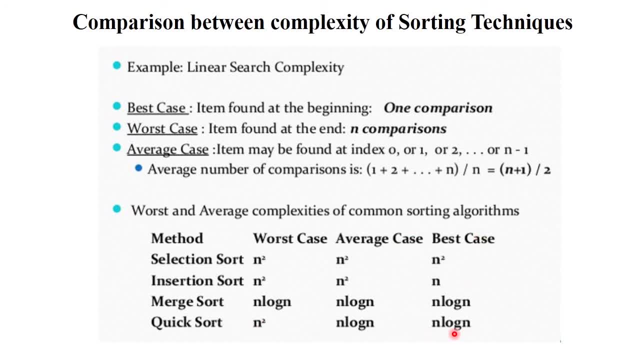 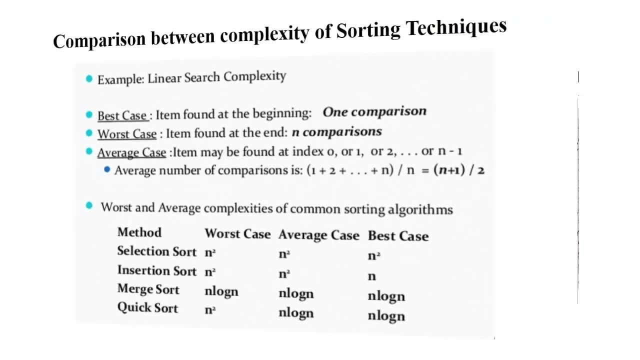 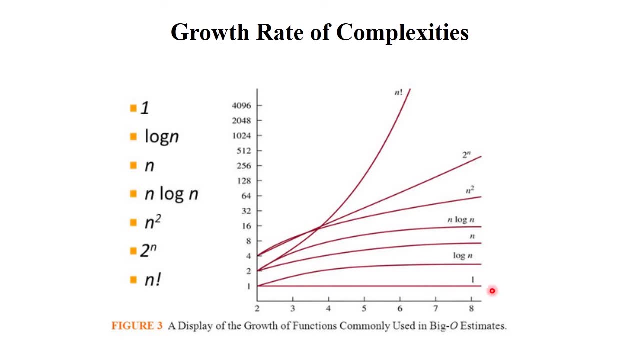 Average and best case is n log, n Clear. So this is one of the most important part in data structure. You have to remember these things Clear Next. So this is just final growth rate of complexities. Okay, The minimum time complexity is declared by the O. 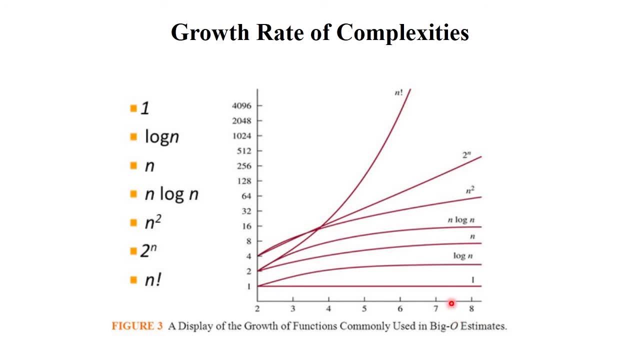 Okay, This is the sequential approach. Okay, The. if the algorithm required largest amount of time, the largest amount of time to solve the particular equation, So it denoted by the n factorial. Okay, This is largest time or maximum time, and is denoted by the minimum time. 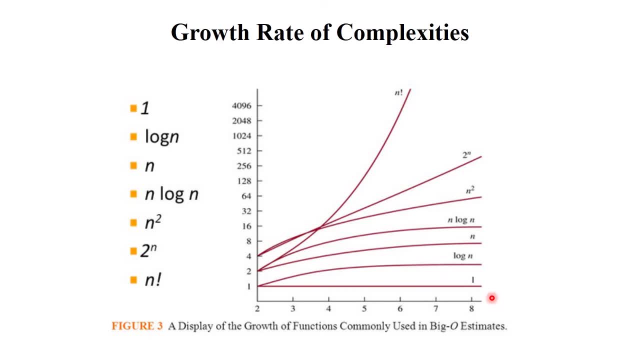 The graph are follow in this way Clear. So sequentially we go. one means shorter time. After that, log n, then n n, log n n square 2 to the power n and at last there is n factorial. This is sequential. 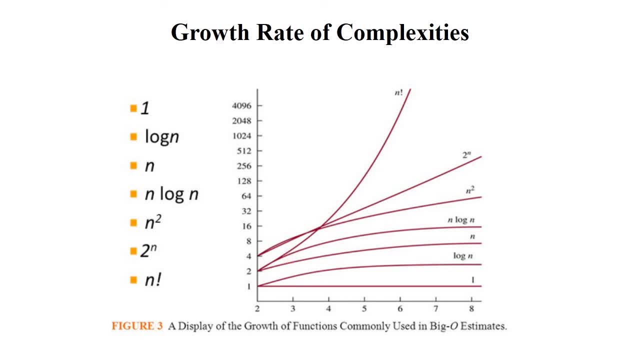 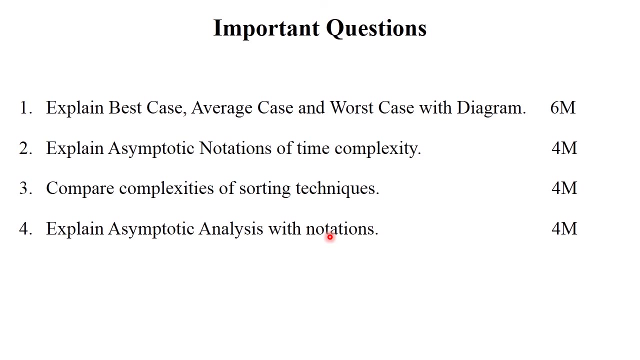 Okay. So while implementation purpose, always we remember the one thing: Your project required minimum time to solve the particular equation or for implementation Clear. Next, These are the some important questions which frequently asked in SPPU exam pattern, like explaining their asymptotic analysis, their notation, comparison of complexities, etc. 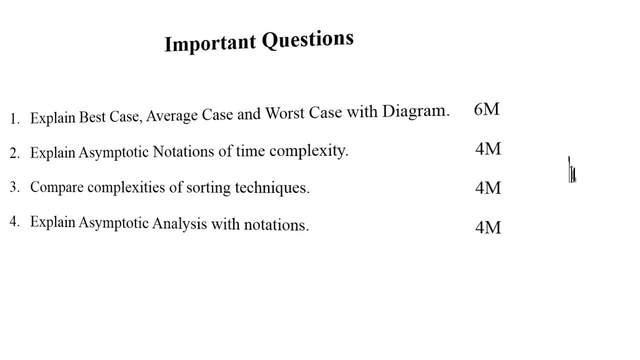 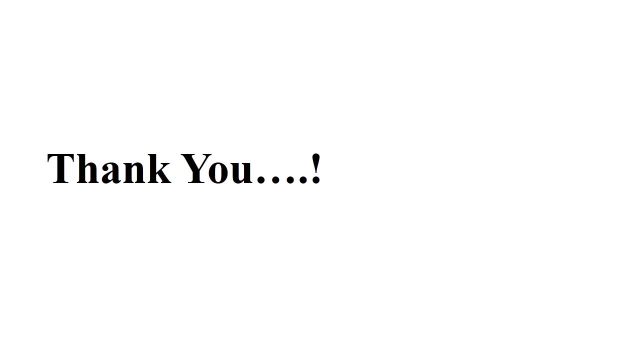 Okay, For this marks Next. So hope so. you understood about space complexity, time complexity, their asymptotic analysis and asymptotic notation. Keep practicing, Thank you.